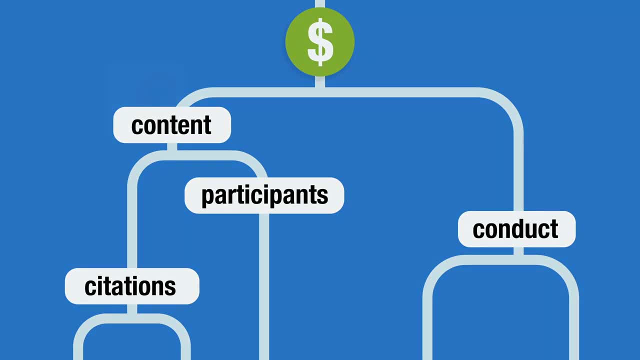 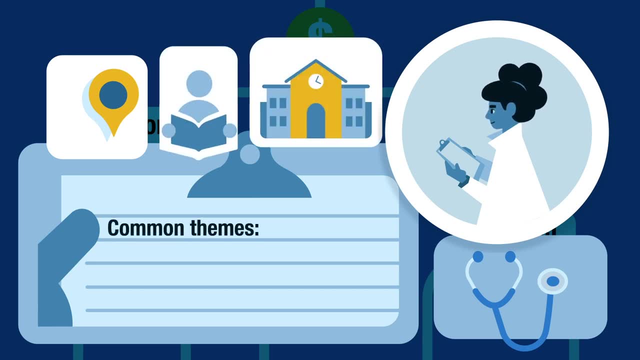 Ethics are even important when examining the sources of funding. Even though ethical standards can vary by region, discipline or institution, there are common themes that determine what makes research ethical. Being honest, transparent and respecting confidentiality and intellectual property are some examples. Different organizations often have their own codes of ethics, For example. 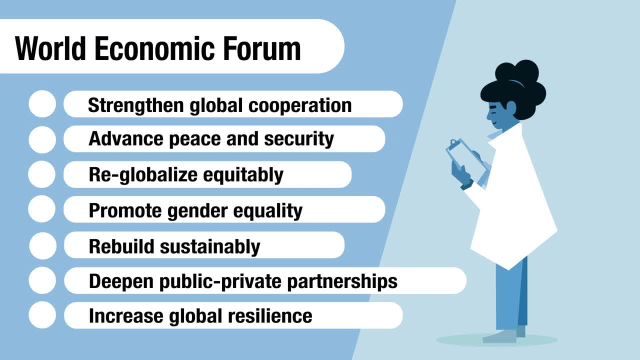 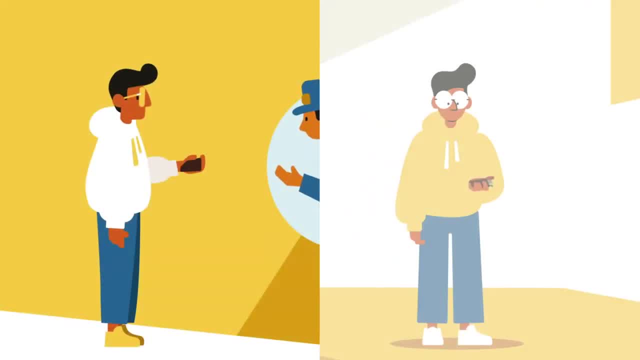 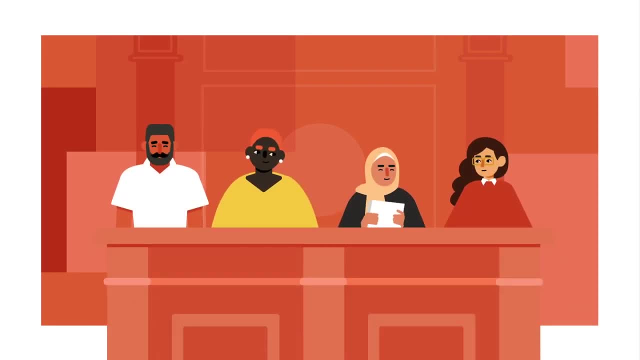 the World Economic Forum Young Scientists Community lists seven key principles for achieving ethical research. Who decides what is ethical and what is unethical? In academia and industry, ethics committees are responsible for reviewing research proposals, monitoring their implementation and following up on their results. Committees have the authority. 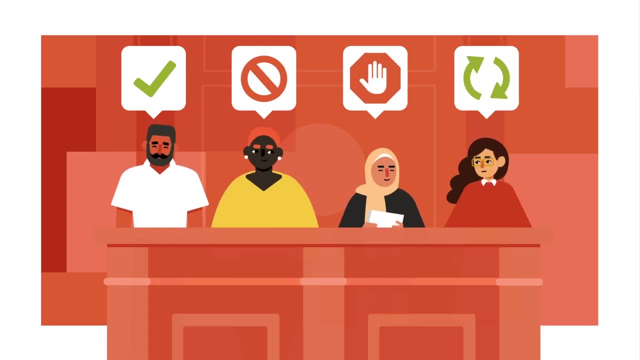 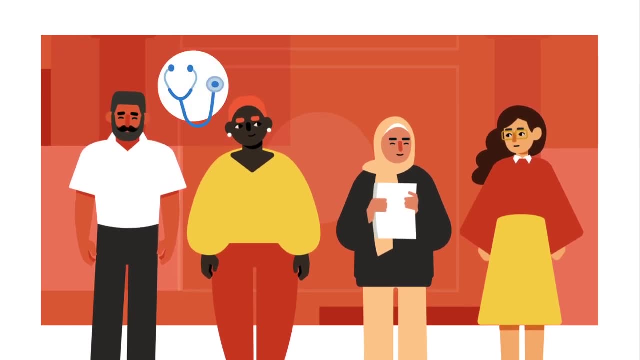 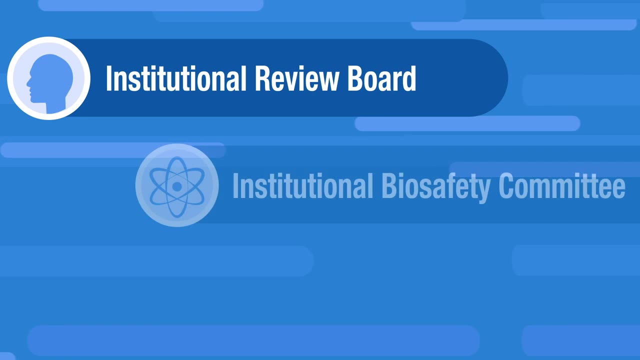 to approve, reject, halt or modify studies if they determine the research to be unethical. These committees consist of people from different backgrounds- scientists and non-scientists alike, to offer different perspectives on ethics. There are different types of committees, depending on whom. 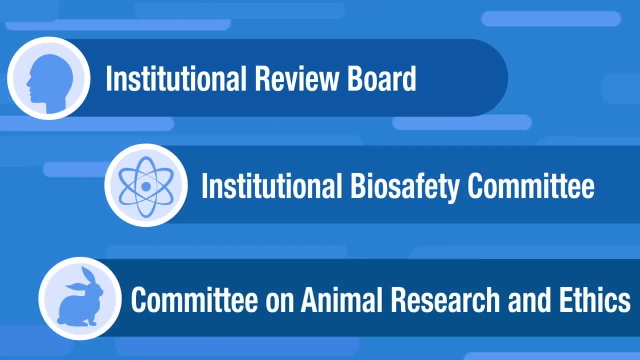 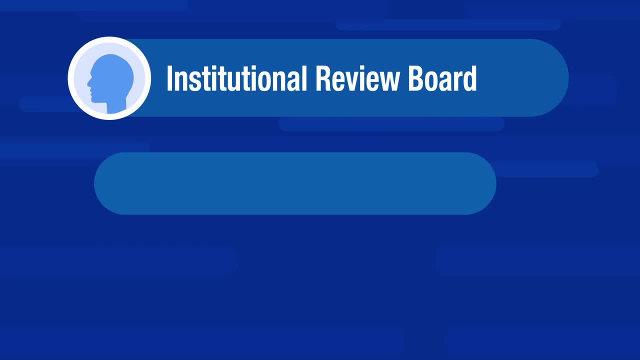 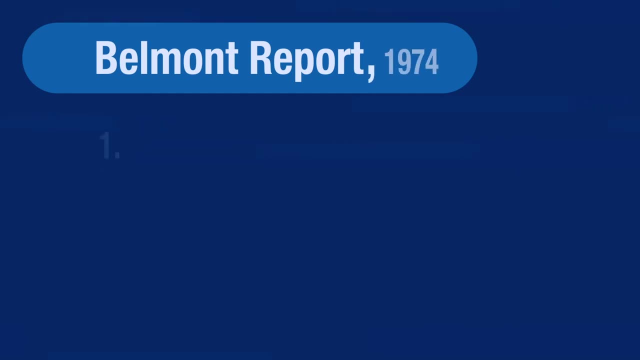 or what is involved in the study. Committees make ethical decisions based on certain principles For research with human subjects. the Institutional Review Board uses the Belmont Report as the foundation for its decisions. The Belmont Report, created in 1974, lists three key 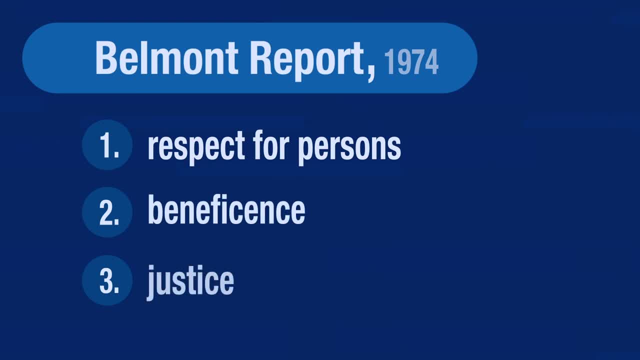 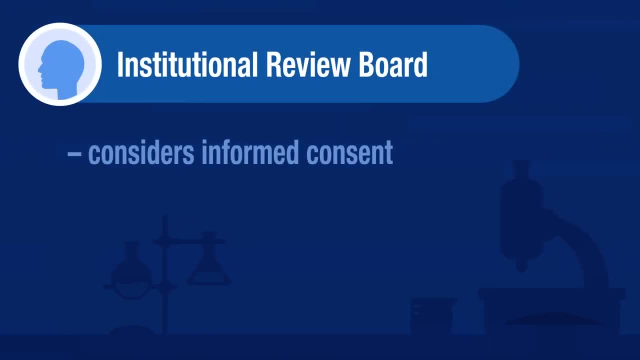 principles: Respect for persons, beneficence and justice. By putting the principles of the Belmont Report into action, the Institutional Review Board considers informed consent to make sure participants understand what they are asked to do for the study, evaluates the potential risks compared to the potential benefits and judges that the selection of participants is fair. 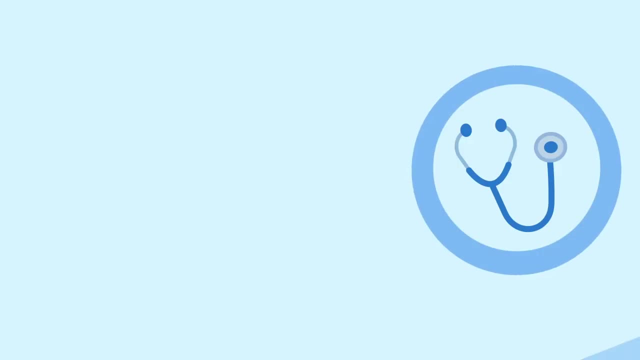 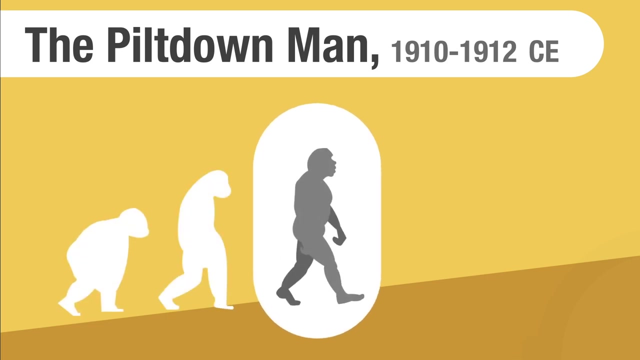 with special protections for vulnerable populations. While there are ethical guidelines in place, unethical research can still happen in any discipline. The Piltdown Man, one of the most famous frauds in archaeology, was accepted as the missing evolutionary link between apes and early humans for decades. 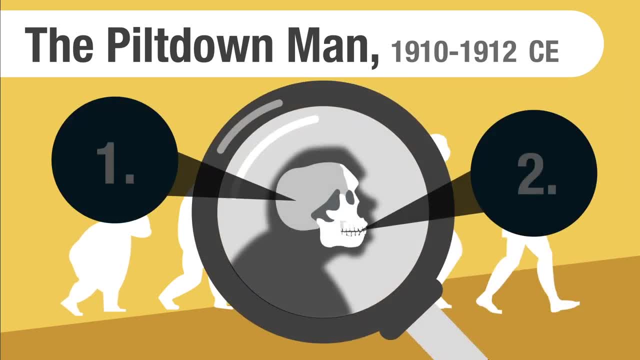 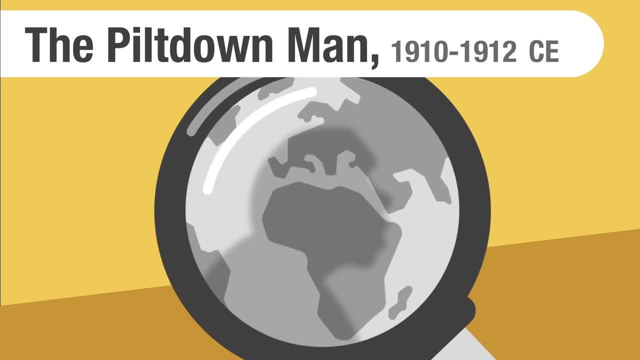 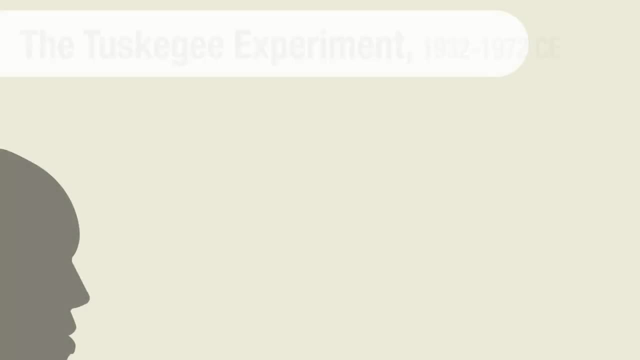 However, the remains were actually from two known species filed and stained to look like a new one. This dishonesty discredited accurate findings of early human remains in Asia and Africa, delaying the process of understanding human history. Another example: the Tuskegee Experiment. 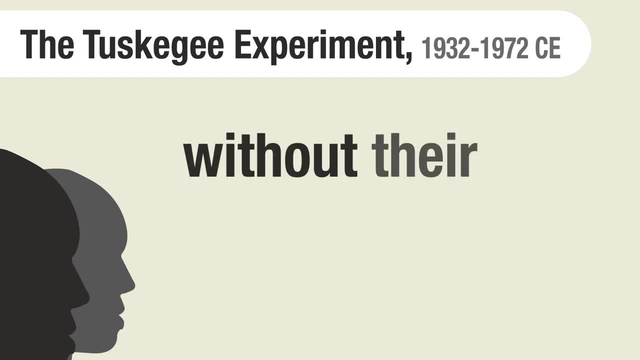 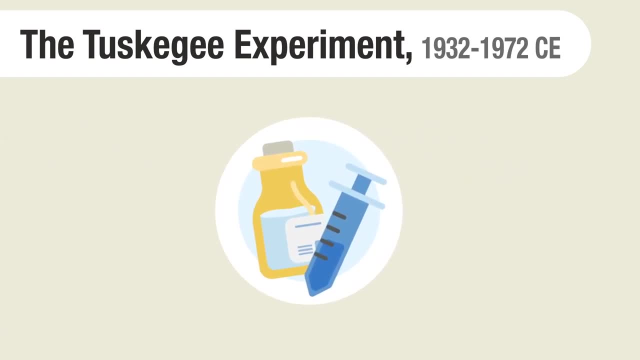 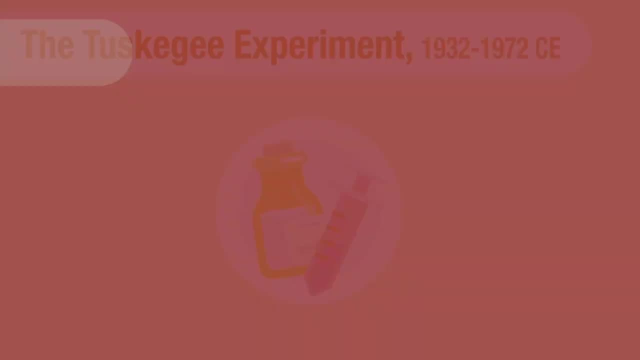 was designed to study the effects of syphilis in black men without their informed consent. Even after penicillin became a known cure for the disease, researchers did not provide adequate treatment to their participants, who eventually died or experienced severe long-term health problems as a result of syphilis. Finally, the MONSTER study was conducted at the University. 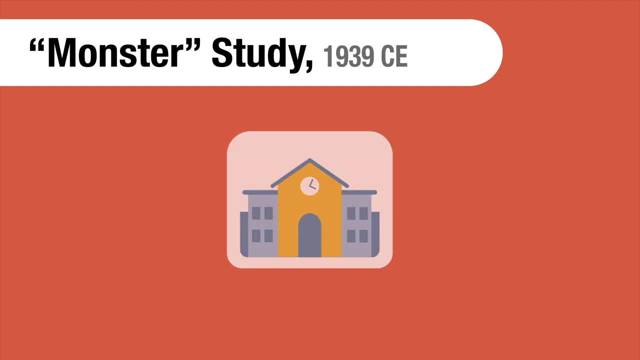 of Iowa to find a cause or cure for stuttering. Twenty-two orphaned children, who were unaware that they were participants in this study, were given either positive speech therapy, which included praise, reassurance and encouragement, or negative speech therapy. 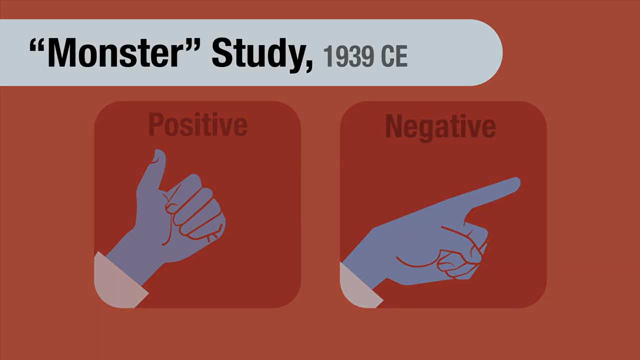 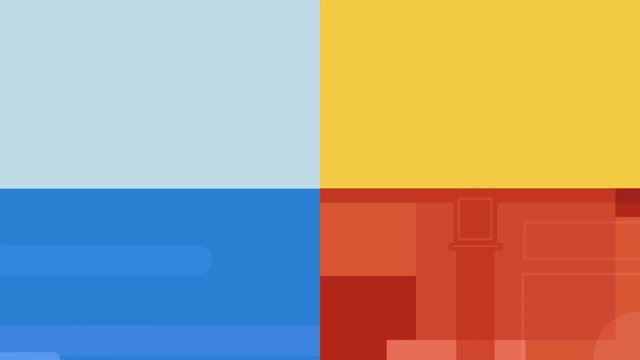 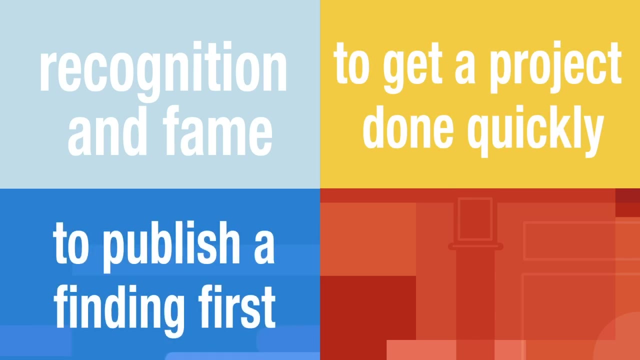 which included belittlement and immediate criticism. Some of the children who received negative speech therapy retained speech problems throughout their lives. There are different reasons why unethical research occurs. It may be motivated by a desire for recognition and fame, to get a project done quickly, to publish a finding first. 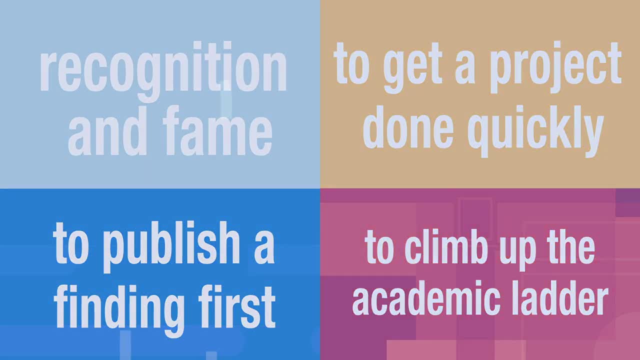 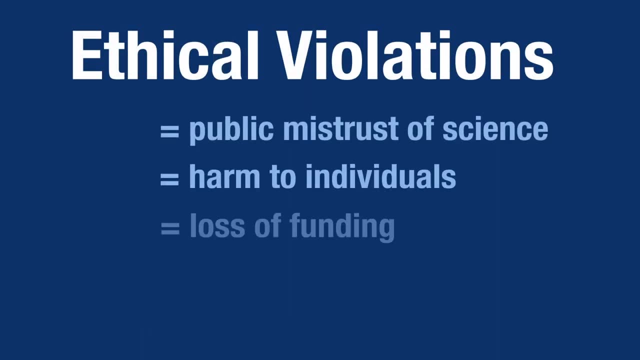 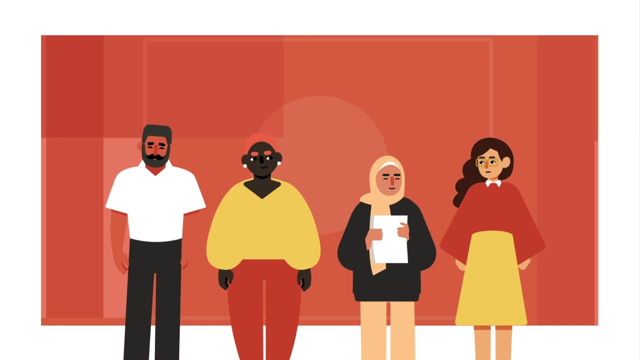 or to climb up the academic ladder. Prejudices and biases may also lead to ethical violations. Public mistrust of science, harm to individuals, loss of funding and even the loss of jobs are some of the consequences of unethical research, While some of the effects of unethical research 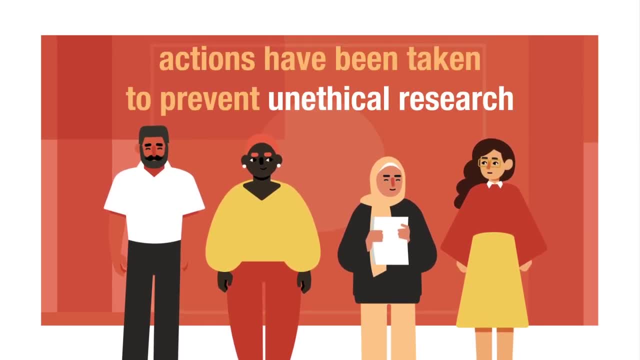 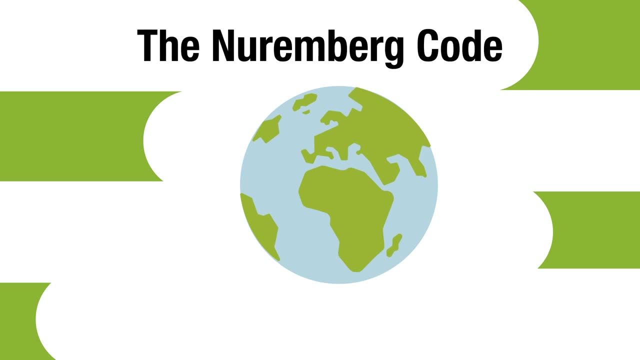 can't be undone. actions have been taken to prevent unethical research from happening in the future. For instance, the crimes against humanity during World War II brought about the Nuremberg Code, the first international document to advocate for informed consent and voluntary participation. 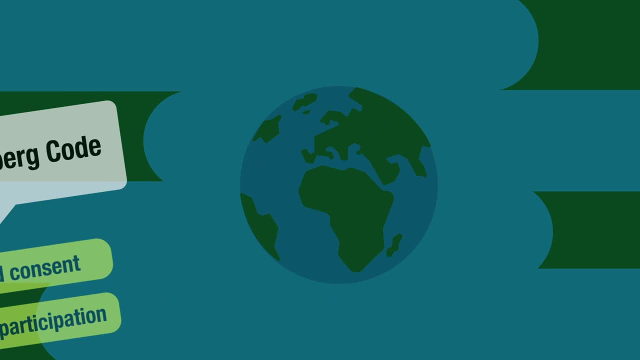 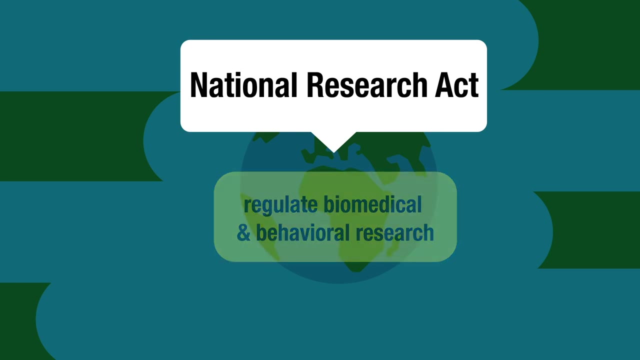 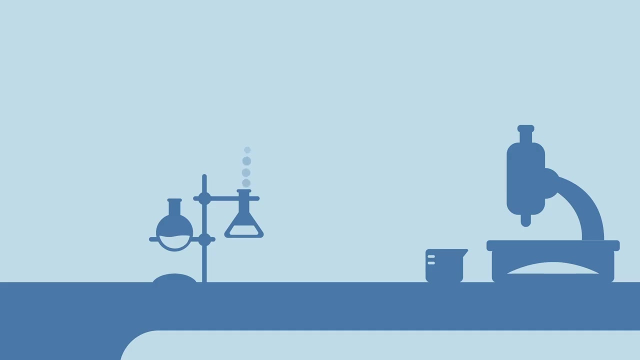 in research involving human subjects. Because of the Tuskegee Experiment, the United States passed the National Research Act to regulate biomedical and behavioral research. The committee created by the act was also responsible for writing the Belmont Report. Today, ethical questions continue to shape. 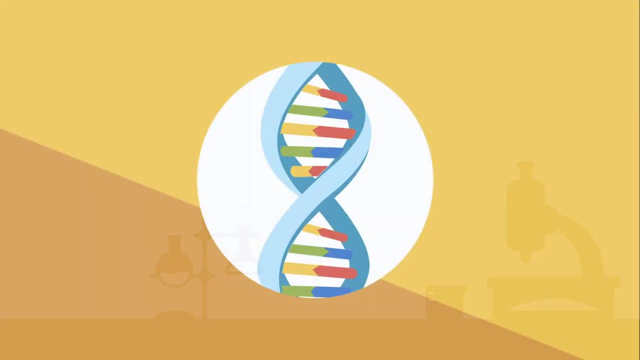 the way we think about research. Consider gene editing a modern innovation to explore some of these questions? By altering our DNA, do we risk creating a modern-day eugenics movement by breeding out undesired genes? Is genetic data private enough to protect personal information? 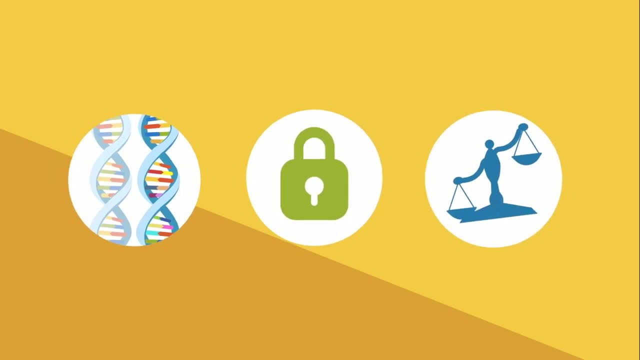 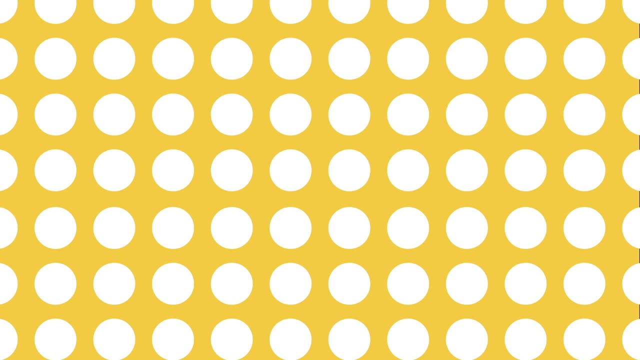 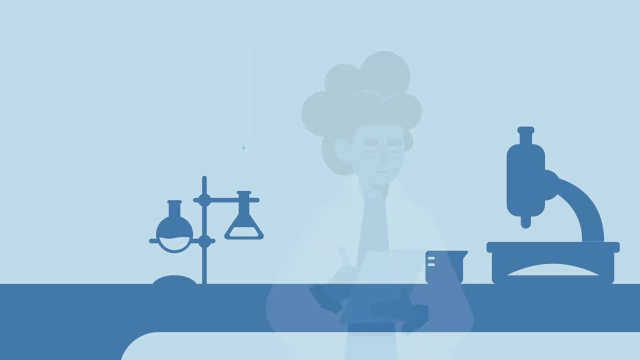 Will gene editing worsen social inequalities? This is not an exhaustive summary of the many roles ethics play in research and the many topics researchers must consider. Ethical training, such as courses and workshops, prepares current and future researchers to work in their desired discipline With the knowledge.